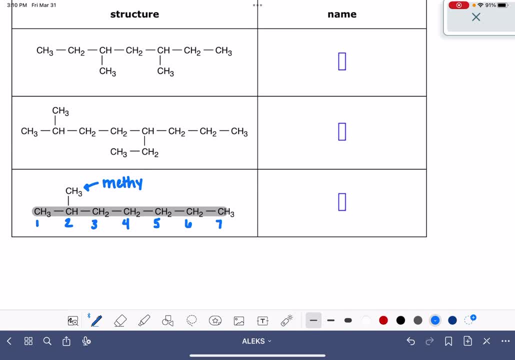 left to right, so that our substituent, methyl, is located on carbon number two. If I numbered from right to left like this, our substituent would be located on carbon number six. And again, we want our substituents to have the smallest possible location Once we have our 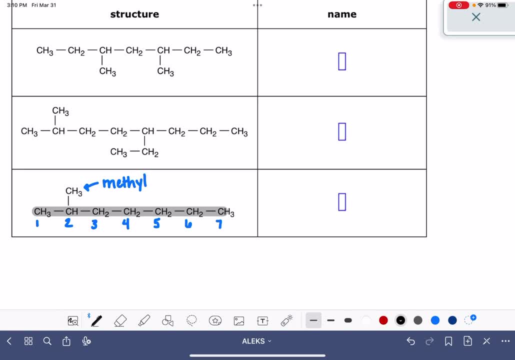 carbon chain numbered and we have our substituents named. we're going to put the molecule's name together. We're going to start by locating and naming our substituents. We have one substituent named methyl and it is located on carbon number two And we indicate that by writing the location. 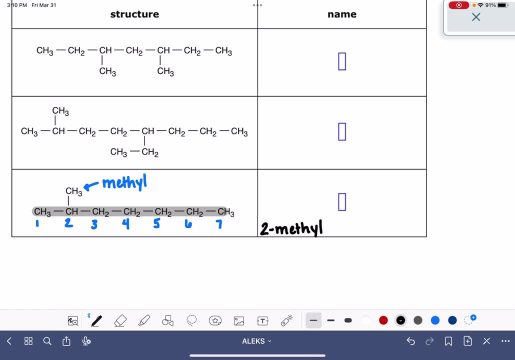 followed by a dash, and then the substituent's name, And then after that we name the parent chain. This is a seven carbon parent chain, and a seven carbon chain is heptane. Let's go up to the first molecule in this problem: Our longest. 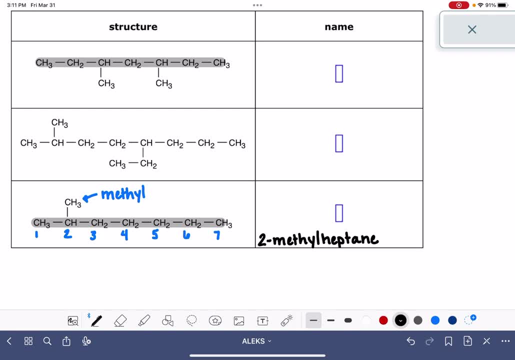 continuous chain of carbons is right here And we are going to number from either left to right or right to left, so that our substituents will have the smallest possible set of numbers. If we go from left to right, our substituents are on carbons three and five. If we go from right to 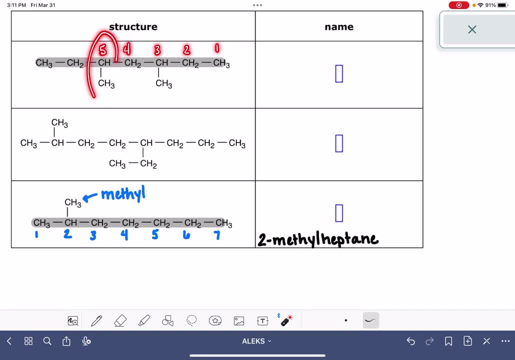 left, our substituents are still on carbons three and five. If we go from left to right, our substituents are still on carbons three and five. In this case, it means it doesn't matter if we number left to right or right to left. I'm just. 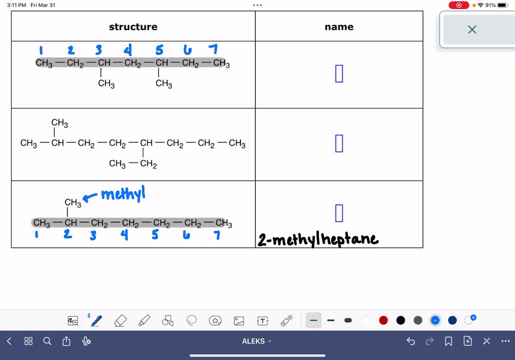 going to go left to right like that. Once we have our carbon chain numbered, we can locate and name our substituents. We have two identical substituents, two methyls. When we have two of the same substituent, we use the prefix di to indicate that we've got two of them. Now we're ready to put. 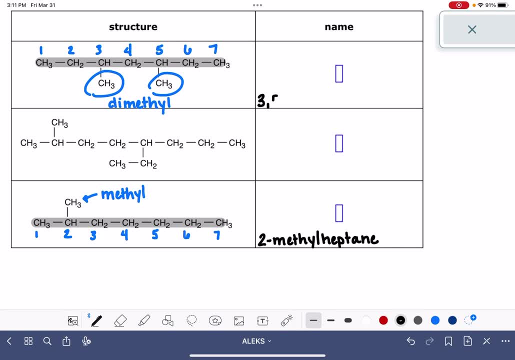 the molecule's name together. Our substituents are located on carbons three and five. We're going to separate the numbers. three comma five say the substituent's name, including the quantity dimethyl, and then the parent chain, which is another heptane seven carbon parent chain. 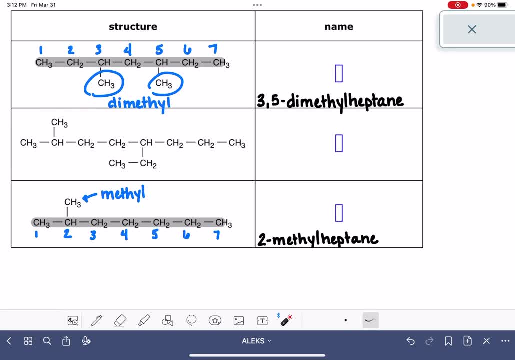 Now, last but not least, we have this one right here. Now this one. I'm not super confident that this is the parent chain. I think that this is the parent chain, but because it's got kind of a funky branch here, I do want to count and make sure that I am choosing the right one. So I'm going to 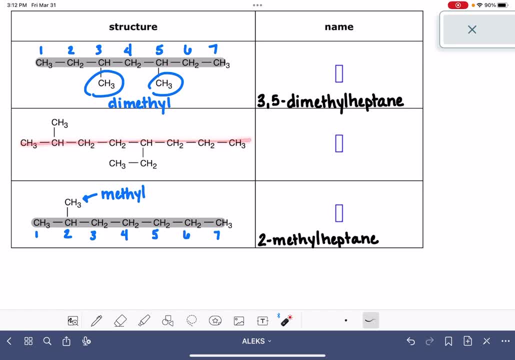 the longest chain of carbons. If this is my parent chain, that is one, two, three, four, five, six, seven, eight carbon chain. Let's just double check this right here. That would be a one- two. 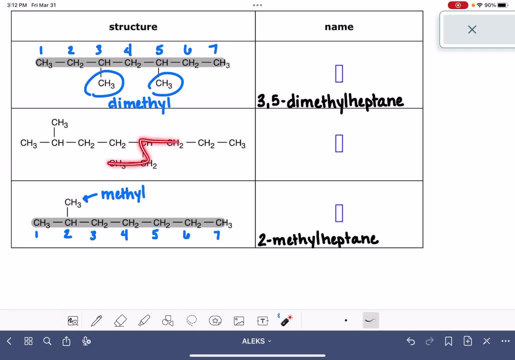 three, four, five, six, seven. Let's double check this: One, two, three, four, five, six. Okay, so this is our longest parent chain. It never hurts to check. We want to number so that our 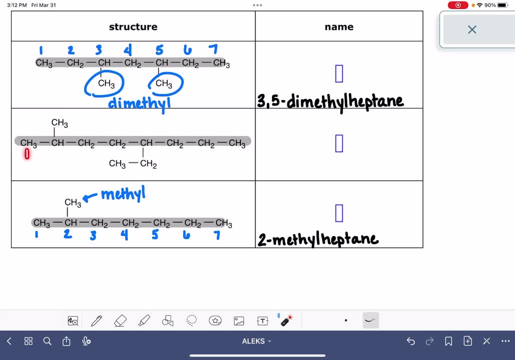 substituents have the smallest possible number, And I think that we're going to accomplish that. left to right, One, two, three, four, five. That puts our substituents on two and five. If we go the other way, yeah, that's definitely not what we want to do. 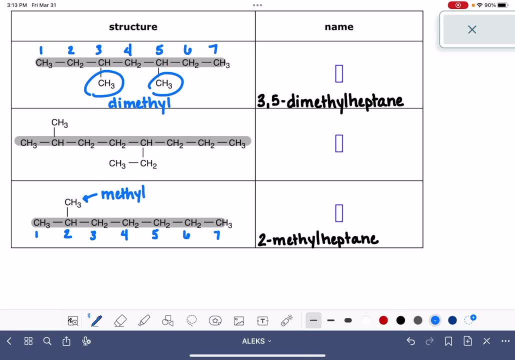 This way would put them on four and seven, So we want to number from left to right: One, two, three, four, five, six, seven, eight. We have a two carbon substituent which is ethyl. We have a. 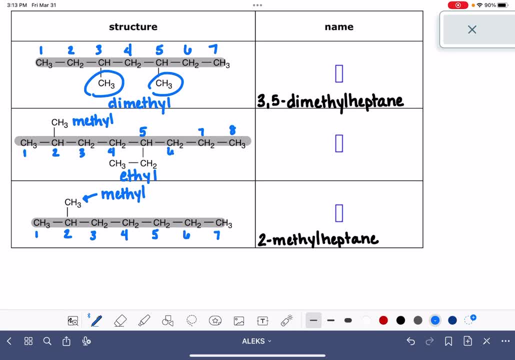 one carbon substituent, which is methyl. When we're putting the molecules named together, we alphabetize our substituents. Ethyl comes before methyl, alphabetically, So ethyl is going to come first in the molecule's name. Ethyl is, on carbon, number five And we're going to follow. 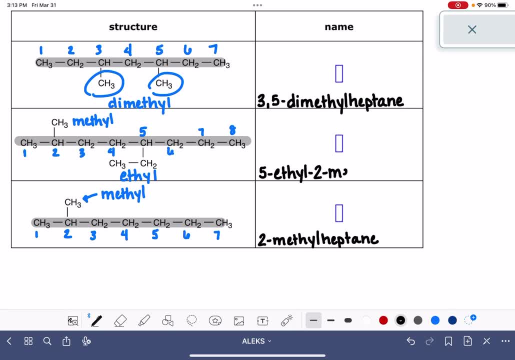 that up with the methyl on carbon. number two: When we're naming molecules, we always use commas to separate numbers from each other And we always use dashes to separate numbers from letters And we put no spaces anywhere in the molecule's name. Now this name for a lot of students, at least initially, is counterintuitive. A lot of students. 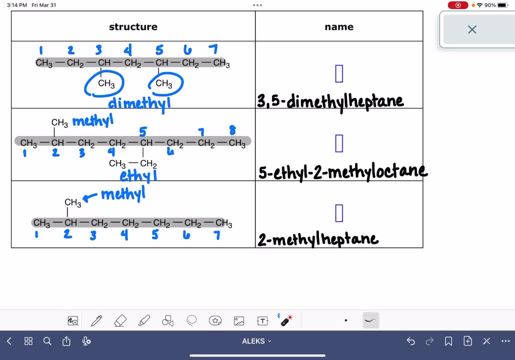 think that they should put the substituents together in terms of numbering priority. So the methyl should have come first in the name because it's on two and the ethyl should come second because it's on five. And that's logical. but it's not how we do it. We put them in. 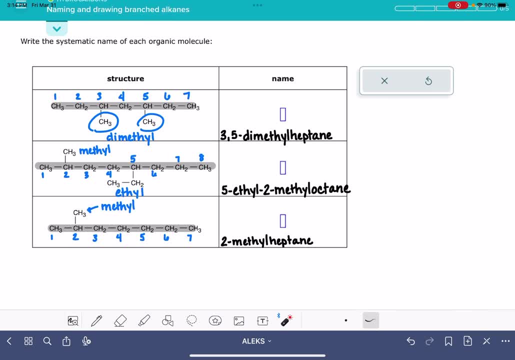 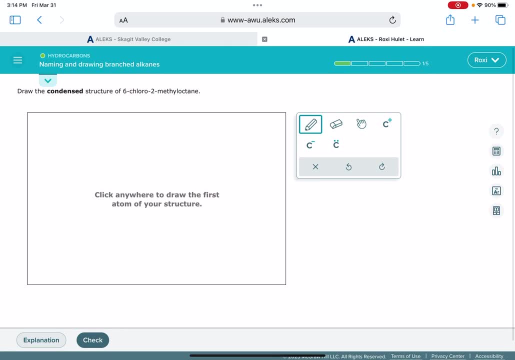 alphabetical order. Okay, so this is one version of the problem where we're naming The other version of the problem. we're going to be given a molecule. We're going to be given a molecule. We're going to be given a molecule's name and asked to draw it, And let's go check this out in. 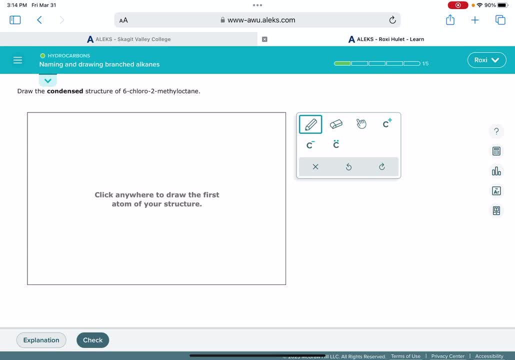 Alex. So this is the other version of the problem. It's asking us to draw a condensed structure, not a line structure of six chloro, two methyl octane. Now, when I'm drawing a molecule from its name, I always start with the ending of the molecule's name first. That is an octane, That's. 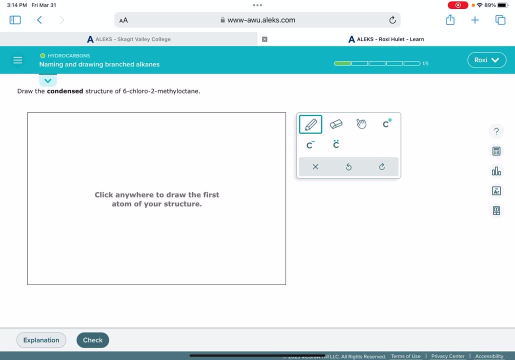 what I want to start with. So I want to make an eight carbon chain for octane, And so I am just going to- okay, be careful, I am going to put eight carbons together in a row like this, And Alex is going to make me do one carbon at a time. What am I up to? One, two, three, four, five, six. 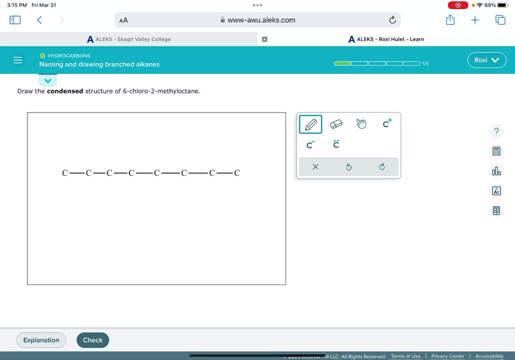 seven, eight. One, two, three, four, five, six, seven, eight. There's my eight carbon chain. Now I'm going to put the substituents on the carbon chain. So I'm going back to the beginning of the molecule's name. It tells me I have a carbon chain. I'm going to put the substituents. 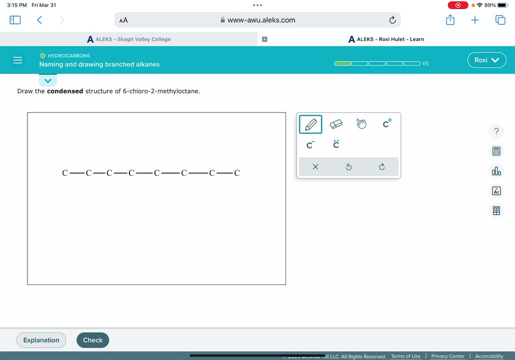 on carbon number six, a chlorine. So I'm going to find carbon number six, one, two, three, four, five, six. I'm going to put a chlorine right there And then it says two methyl. So that means on carbon number two I have a methyl which is a CH3. Now, this is not. I'm not done. 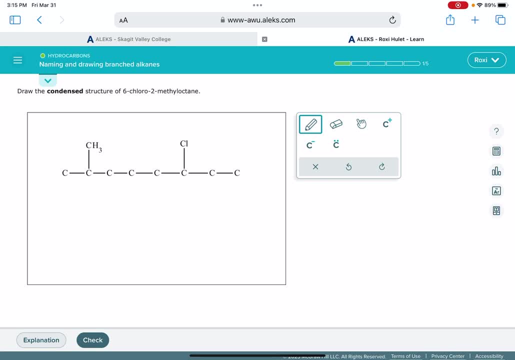 This isn't it. I'm not done My parent chain. I started by just putting carbon atoms down, but those carbon atoms have hydrogens on them and they need to be there In order for this problem to be correct. So I need to go back and change all of these carbons. 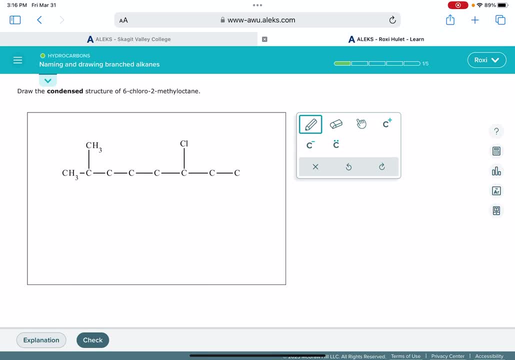 to the correct group, CH3.. My second carbon, carbon number two. right now. it only has three bonds, So that means I need to have a hydrogen on there, So that needs to be a CH. The next one is a CH2.. Actually, the next few are CH2s. This one is a CH, There's another CH2 and there is my CH3.